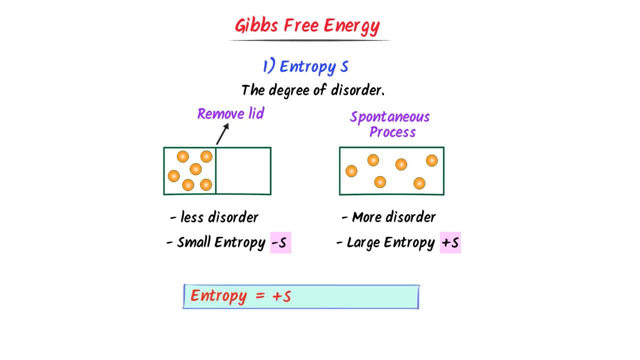 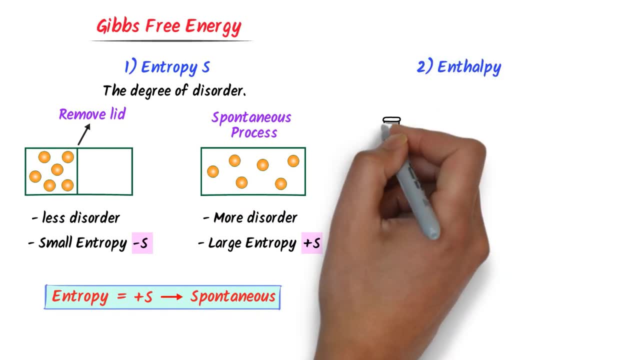 we learn that if entropy is increasing or positive, it is a spontaneous process. Secondly, understanding enthalpy. Let's consider this hot water and this speaker. We know that entropy is increasing or positive, Hence its entropy S is also high or its entropy S is. 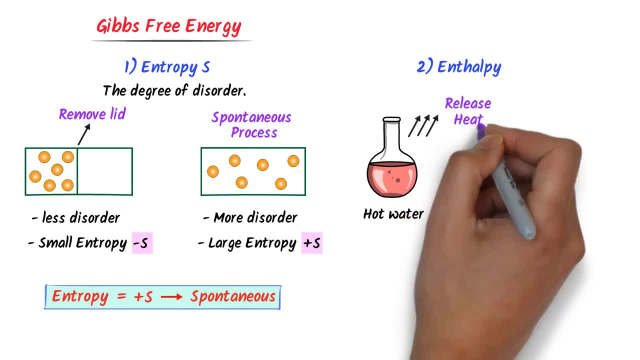 negative. We know that with the passage of time, hot water releases heat into the surrounding. The hot water releases heat so that it gains stability. We know that when a system releases heat into surrounding, its enthalpy change, del H, is negative and it is an exothermic process. 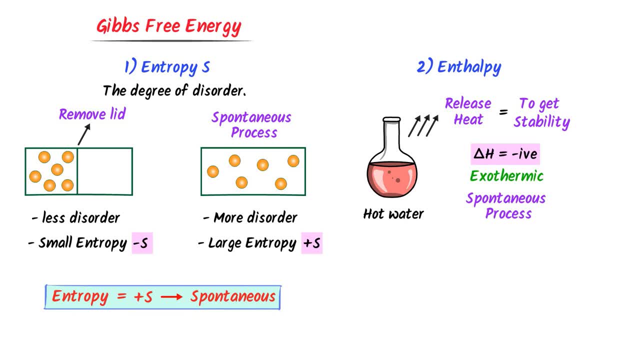 Also, it is a spontaneous process. Thus we conclude that if enthalpy change del H is negative, then it is a spontaneous process. Hence we conclude that if enthalpy change del H is negative, it is a spontaneous process. Thirdly, understanding the effect of 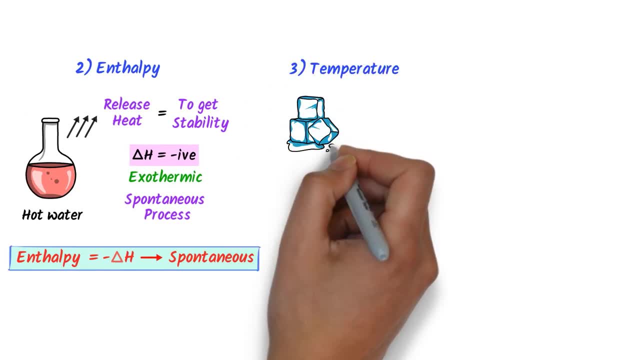 temperature on spontaneous process. Let's consider this melting ice. We know that melting of ice is a spontaneous process. Now, if I add some sort of heat to this melting ice, it will quickly melt. Thus we conclude that if we increase temperature, the rate of spontaneous process either increases- 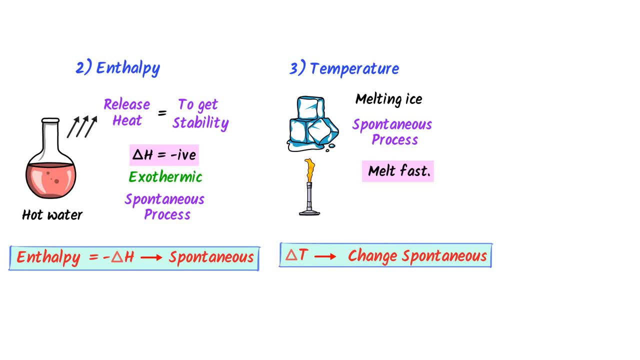 or decreases. So if we increase temperature, the rate of spontaneous process either increases or decreases. Hence note down all these important points. Until now, we learned that any spontaneous process is affected by enthalpy change del H, entropy del S and temperature T. These three 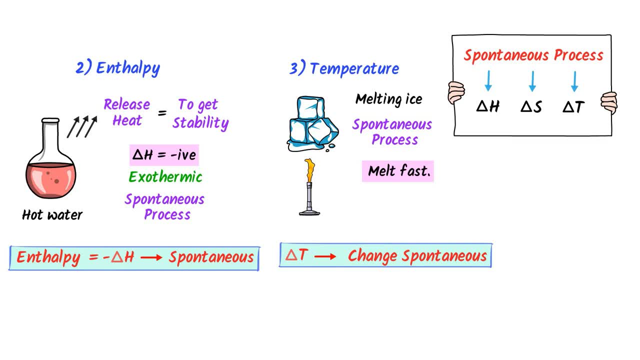 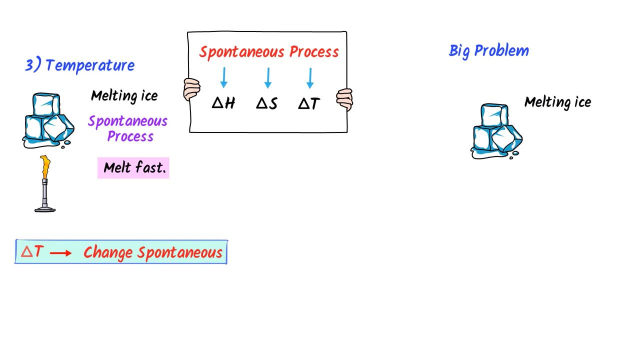 variables are must for understanding any spontaneous process. Now here is one big problem. For example, consider this melting ice. We know that this melting ice absorbs heat from the surrounding and it is an endothermic process. It is also a spontaneous process. Also, we know that for endothermic process, enthalpy change del H is 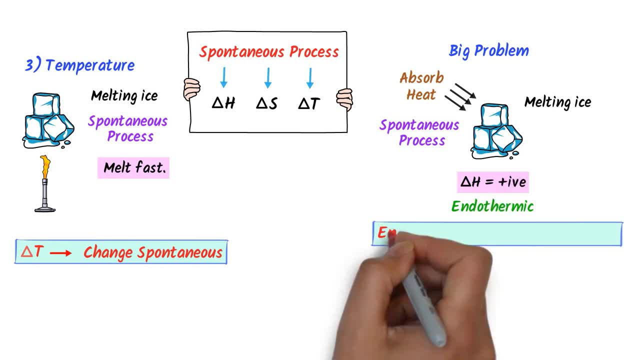 positive. Hence we conclude that if del H is positive, it will be a spontaneous process. But wait a minute, This is a big problem. We already learned that if del H is negative, it will be a spontaneous process, While here del H is positive, but it is still a spontaneous. 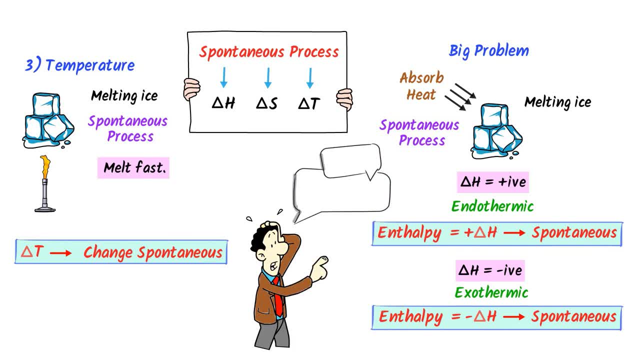 process. Therefore we say that del H cannot show us that a process is spontaneous. Let me repeat it: Del H alone cannot show us that a process is a spontaneous. So I cross it Now. the question is: how can we determine that a process is a spontaneous process? 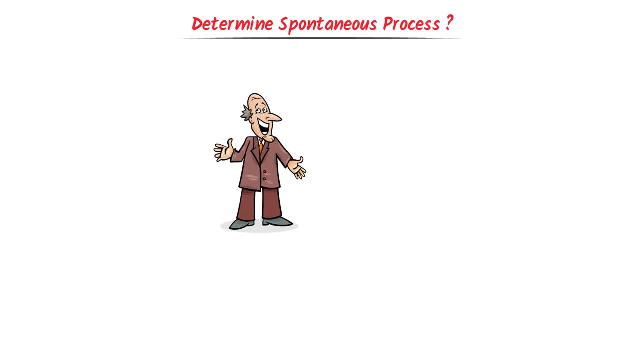 Well, here comes Gibbs Baba. He took a blender and added del H, T and del S to it. He formed a mixture of del H minus T del S. He called this mixture as Gibbs free energy. It is denoted by del humble g, Hence Gibbs free energy tells us whether a reaction 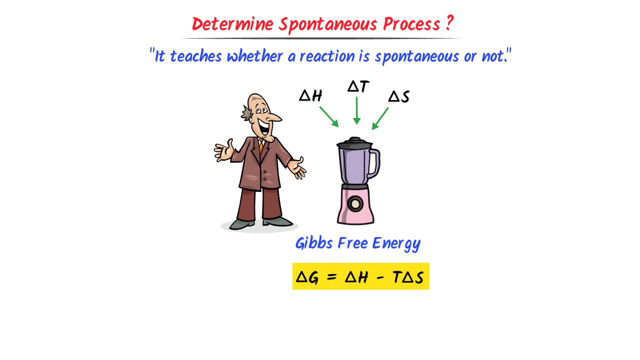 is spontaneous or not. Let me repeat it, Gibbe, free energy is a variation of a state of, So such a reaction takes place when a response is spontaneous. and we multiply the given Brentrin and delta S, We say that these two appetizers, as well as theihen, give rise to seismic energy. 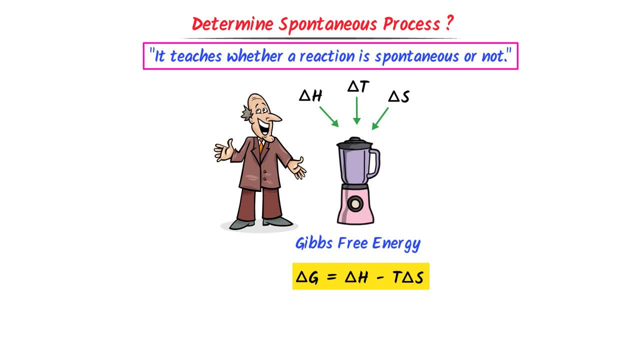 energy tell us whether a reaction is spontaneous or not. Therefore we say that enthalpy change and entropy cannot determine a spontaneous reaction. Rather, it is the Gibbs free energy that determines whether a reaction is spontaneous or not. For example, it shows that if del G is 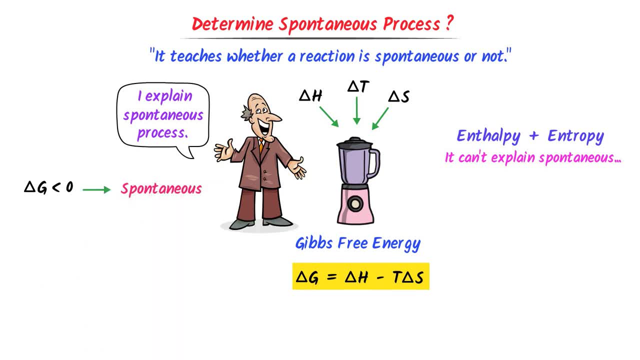 less than zero or negative, it is a spontaneous process. If del G is greater than zero or positive, it is a non-spontaneous process. If del G is equal to zero, it is an equilibrium stage. To remember, Gibbs: free energy. note down this easy mnemonic. 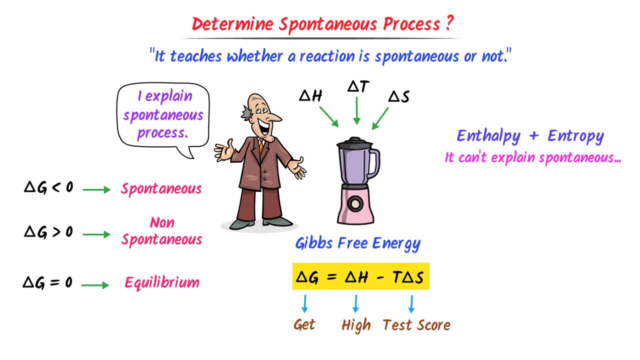 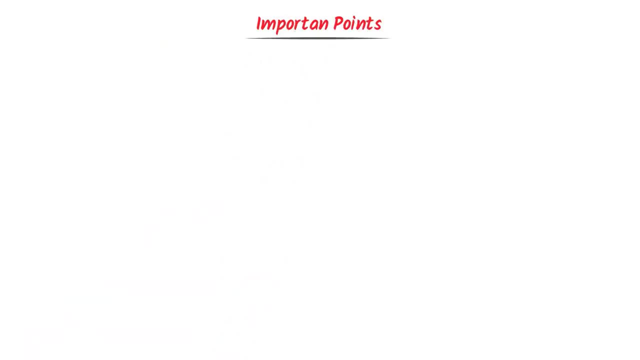 Get high testing score. Let me repeat it: Get high testing score. Therefore, we say that Gibbs free energy is less than zero or negative. it is a spontaneous process. Now let me teach you some important points about Gibbs free energy. We know that del G is less than zero or negative. it is a spontaneous process. 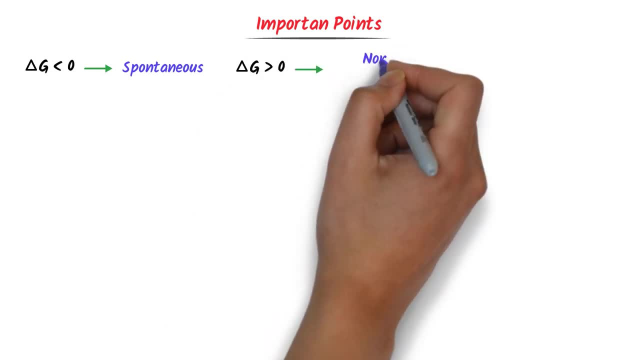 Del G is greater than zero or positive, it is a non-spontaneous process. When del H is equal to zero, it is an equilibrium stage. Now I will prove it in a very easy way. I write here del H and del S. Let del H is negative or it is an exothermic process. 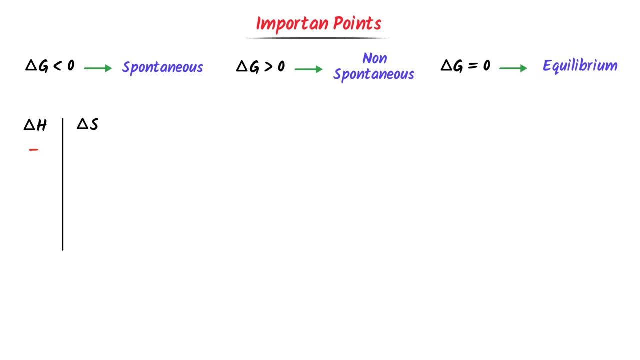 in which heat is released to surrounding. We know that in an exothermic process usually the randomness or disorder of Gibbs molecules increases. Let its entropy, del S is positive. Also, we know that del G is equal to del H minus T, del S. Here. 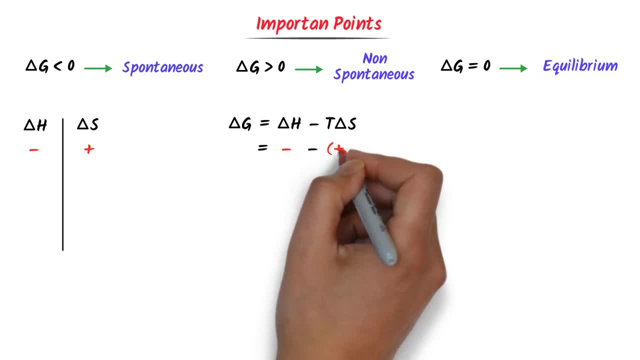 del H is negative, minus del S is positive. This minus and to this positive is equal to negative. I write negative and negative. We know that when we add two negative numbers we get a negative number. So here del G is equal to negative number. Therefore we say that: 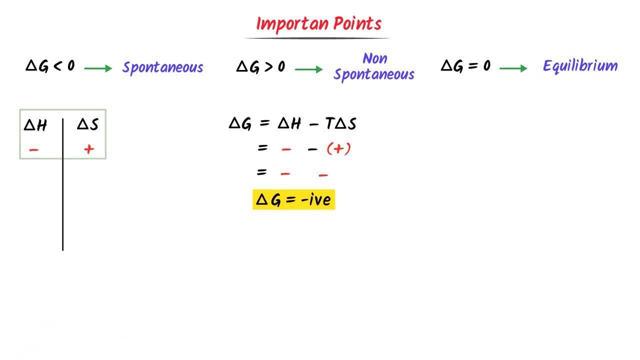 when del H is negative and del S is positive. it is a spontaneous process. Secondly, let del H is positive and del S is negative. We already know that del G is equal to del H minus T into del S. Here del H is positive. 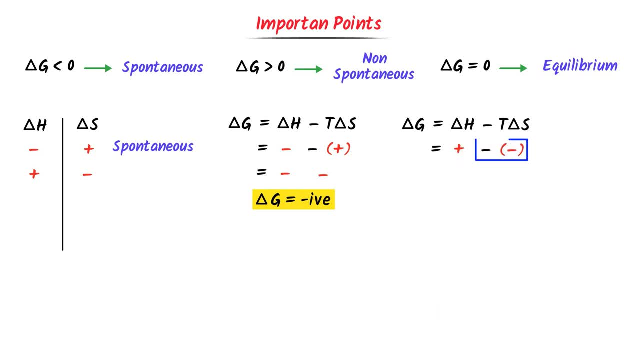 minus del S is negative. Now minus into minus is equal to positive. I write positive and positive. We know that when we add two negative numbers we get a negative number. So here del G is equal to positive number. When we add two positive numbers we get a positive number. So 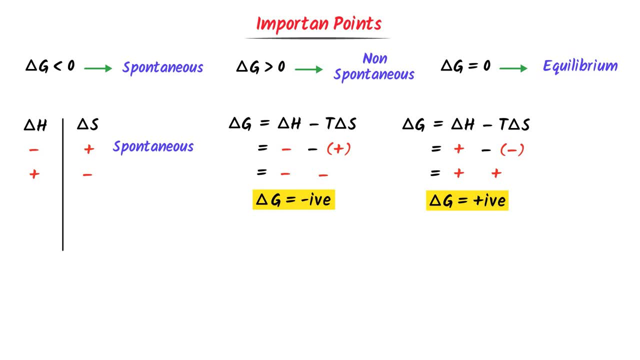 del G is equal to positive number. Therefore, we say that when del H is positive and del S is negative, it is a non-spontaneous process. Now, in the light of this information, consider this important MCQs from competitive exam. A process will be spontaneous at all. 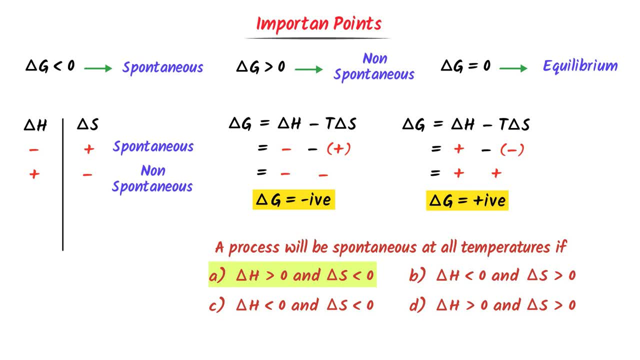 temperatures if del H is got 0 and del s is less than 0.. B option del h is less than 0 and del s is greater than 0.. C option del h is less than 0 and del s is also less than 0.. D option del h is: 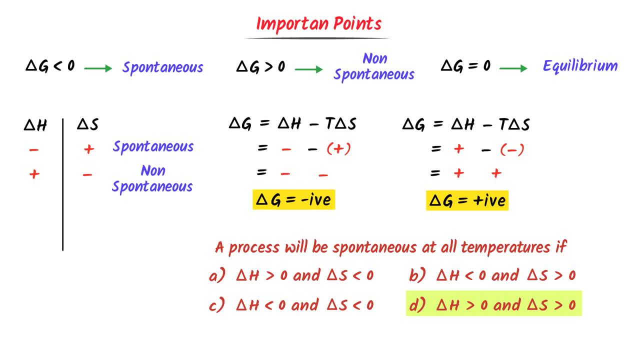 greater than 0 and del s is also greater than 0.. Pause the video and try to answer it Well. Well, we know that when del H is less than zero or negative and del S is greater than zero or positive, then del G will be negative and the process will be spontaneous at all. 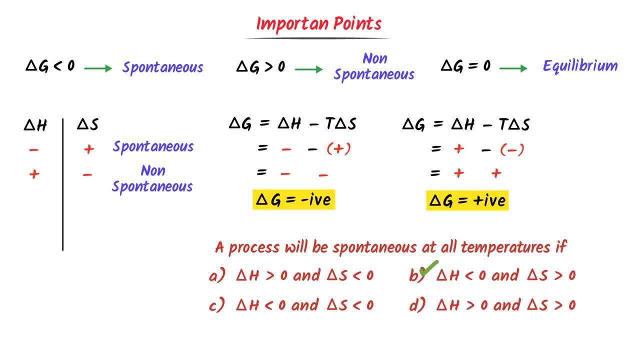 temperature. Hence the correct option is B. Thus note it down. Thirdly, let del H is positive and del S is also positive. We know that del G is equal to del H minus T into del S. Here del H is positive. 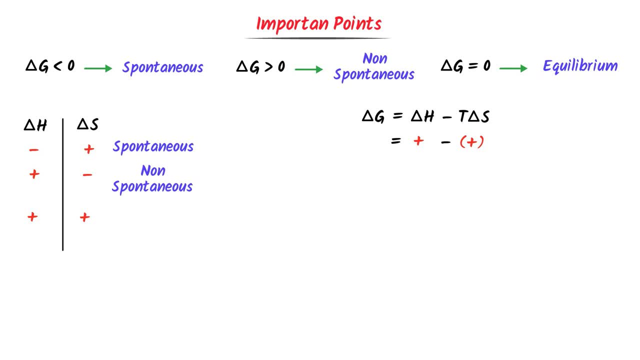 Minus del S is also positive. Minus into plus is equal to minus. I write plus and minus. Now one is positive number and another is negative number. We may get the value of del G as both positive or negative, I mean. 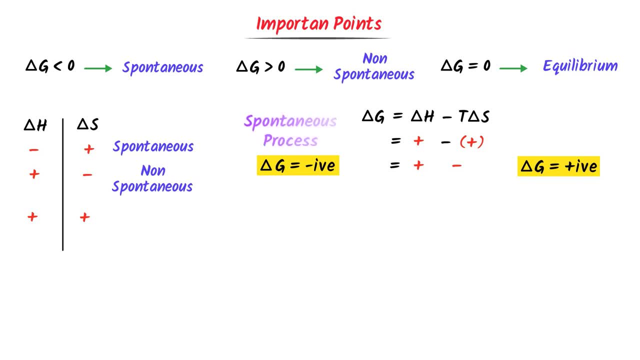 if the value of del G is negative, then it is a spontaneous process. If the value of del G is positive, then it is a non-spontaneous process. We know that in case of spontaneous process, del G is less than zero. 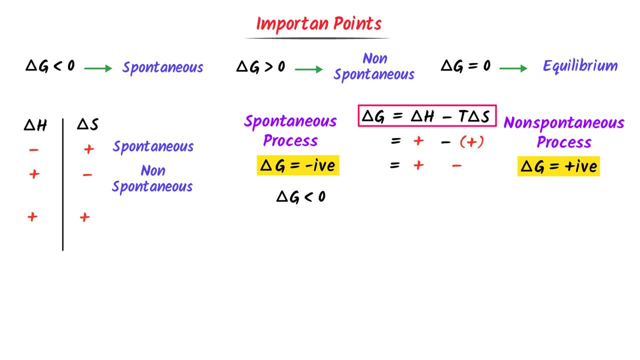 The value of del G is del H minus T del S. I write: del H minus T del S is less than zero. Our T del S is greater than del H minus T del S. Our T is greater than del H upon del S. 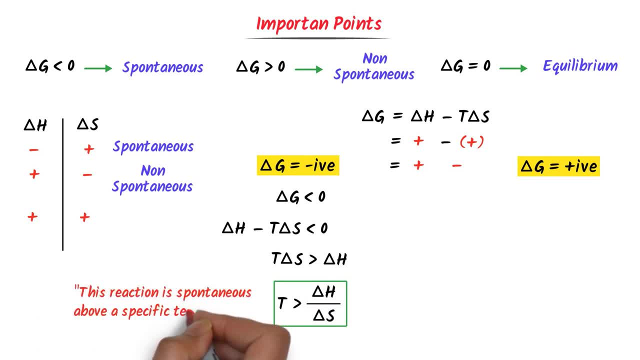 It means that this reaction is only spontaneous above a particular temperature. Let me repeat it: This reaction is only spontaneous above a particular temperature. Secondly, we know that in case of non-spontaneous reaction del G is greater than zero, The value of del G is del H minus T del S. 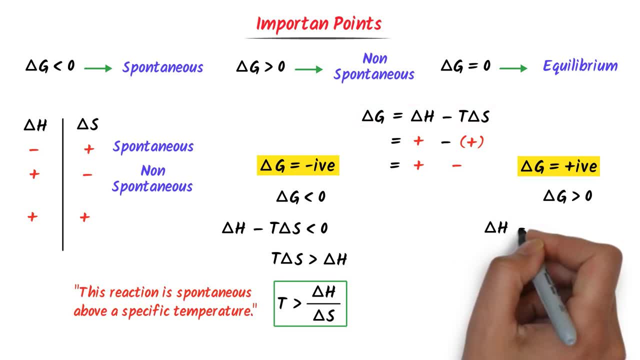 We know that in case of non-spontaneous reaction, del G is greater than zero. The value of del G is less than del H upon del S. It means that this reaction is only non-spontaneous below a particular temperature. We know that in case of non-spontaneous reaction, del G is greater than zero. 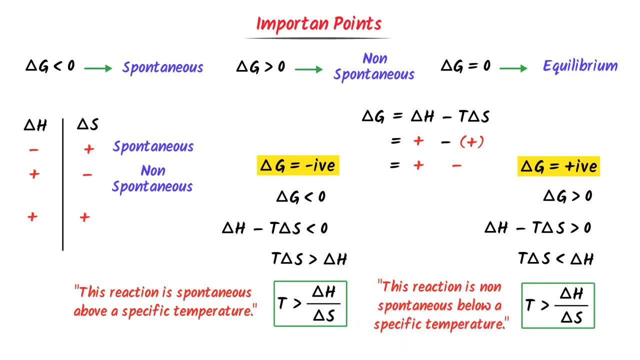 Therefore I write: del G minus T, del S is 0.. Otherwise, del G is non-spontaneous above a particular temperature. Let me repeat it: of del H and del S is positive. the reaction is spontaneous above one temperature or non-spontaneous. 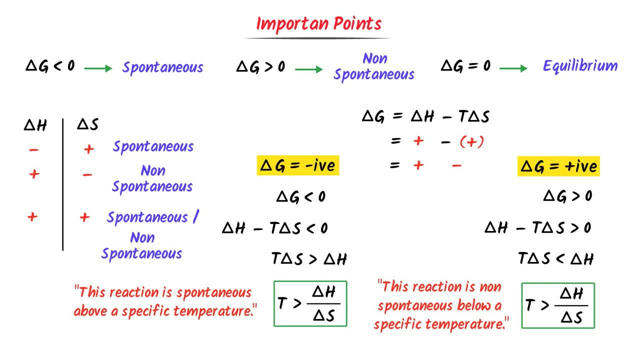 below another temperature. Let me repeat it: If the value of del H and del S is positive, the reaction is spontaneous above one temperature or non-spontaneous below another temperature. Similarly, if to both are negatives, we say that the reaction is spontaneous. 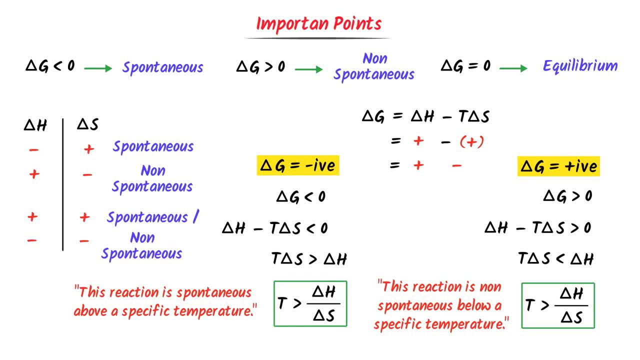 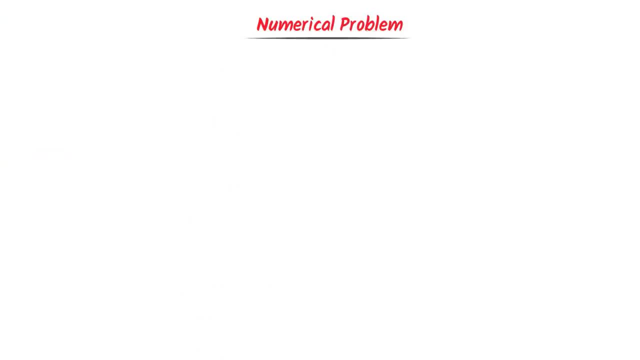 and non-spontaneous at different temperatures. Thus noted down all these important points, Finally, let consider this numerical problem. from competitive exam, The reaction as follows: Del H sú del H 넘ô guardiansur is 491.1 kJ per mole and del S is equal to 198 Joule per kilo mole. It is not feasible at 298. 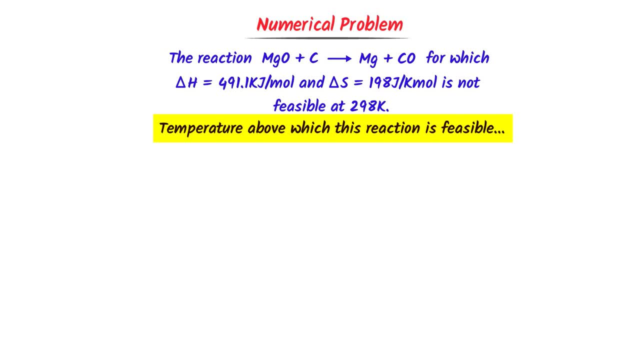 Kelvin Temperature above which this reaction will be feasible is dash. Firstly, I write the given data like: del H is equal to 491.1 kJ per mole, or 491.1 x 103 Joule per mole, and the value of del S is equal to 198 Joule per Kelvin mole. Secondly, the word feasible means 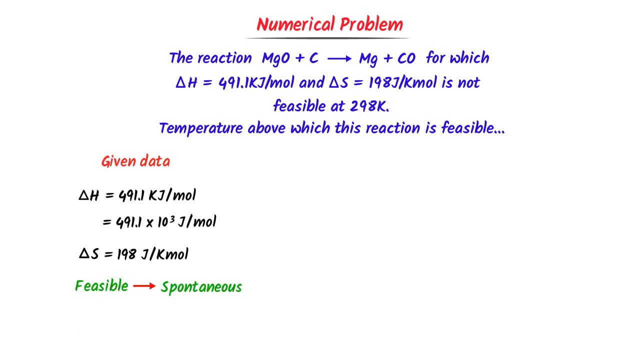 spontaneous. In the question we are asked that above which temperature this reaction reaction will be feasible- are spontaneous. We already know that if del G is less than zero, it is a spontaneous reaction. The value of del G is del H minus T into del S is less. 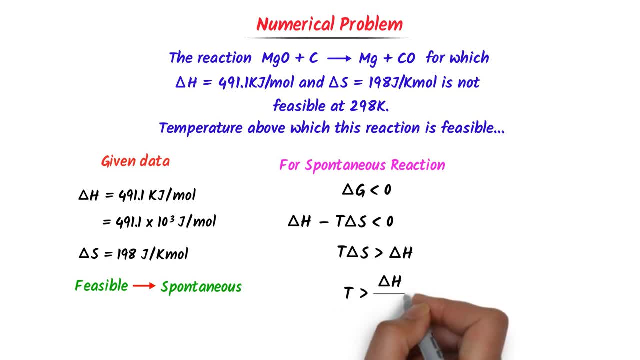 than zero. RT is greater than del H upon del S. I plug in the values of del H and del S in this equation. After calculation I get: T is greater than 2480.3 Kelvin. It means that this reaction is spontaneous at temperature greater than 2480.3 Kelvin. Below this temperature,